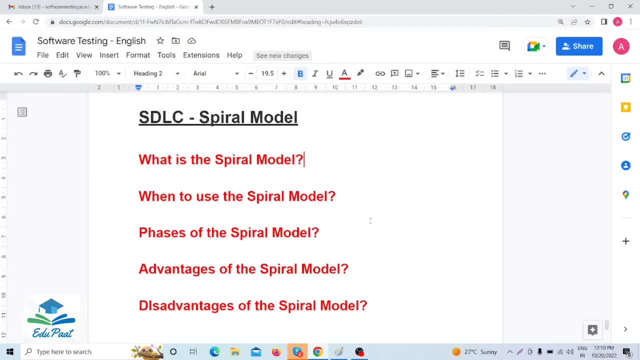 Hello everyone, Welcome back. So today I am going to discuss you SDLC spiral model. I will give you a very easy way that. how can you guys remember that what is spiral model and how it works? So let's start about what is spiral model. 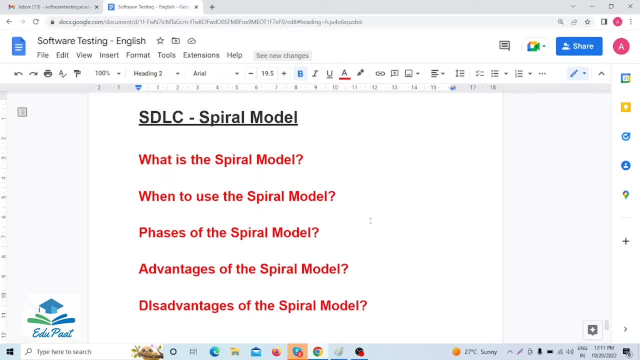 So, guys, if you have remembered that, I have already discussed about the last video, waterfall model. So there I have discussed about the advantages and disadvantages of waterfall model. So if you guys remember the disadvantage of waterfall model, So to avoid that disadvantage or to avoid the drawback of that waterfall model, the spiral models come into the picture. So, basically, what is the spiral model? 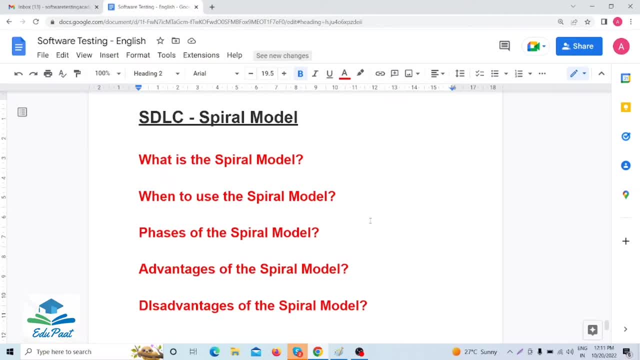 Now I am telling you one by one, So you guys will be better understand that, what will be happening on the spiral model. What is spiral model? Spiral model is a step by step procedure or standard procedure to develop any software. Spiral model is a step by step procedure or a standard procedure to develop any software. So to avoid the waterfall model drawbacks, we use the spiral model. Okay, Now already I have. 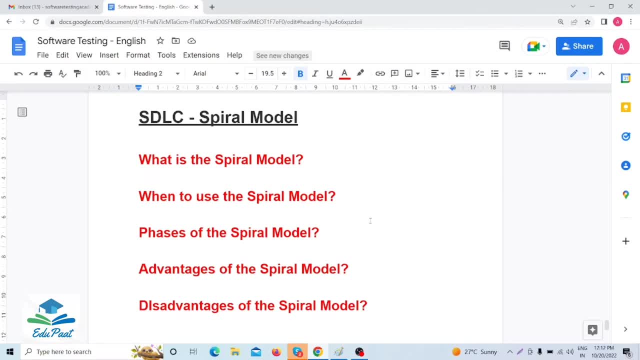 So if you guys already guys, I have already guys, I have told you that in the waterfall model, if you guys remember that waterfall model, if any phases is working- suppose I am working on the feasibility study phase- if any phase is working, then we can actually work. 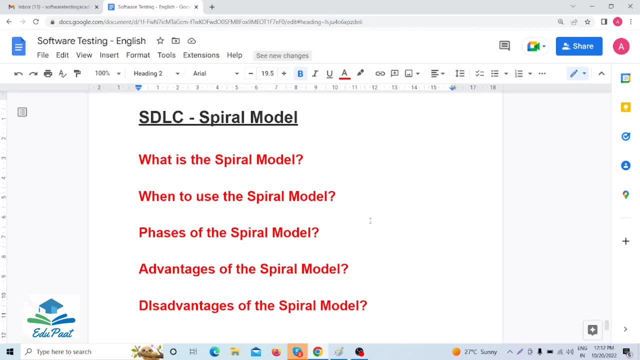 Waterfall model. if any phases is working. suppose I am working on the feasibility study phase. if any phases is working, then can not the previous phase in the waterfall model Right? That means I require, not change the requirement, means requirement will be free Right. Apart from that artifial model. if we say I am working on the feasibility study, makeup is working first, The natural process of that other thanoker. so we cannot change the requirement right, The strata. What we are interested in is потому I'm most interested in the precise unseriousness of pyramidal velocidad. 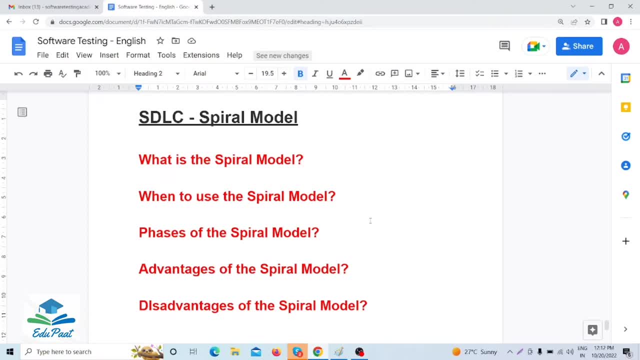 apart from that, in the spiral model, when, when we follow the spiral model, when we use the spiral model, when the, when, the module in that modules, if there is any dependency among with the modules, if there is any dependency. now the question is that what is module? module means we can say that. 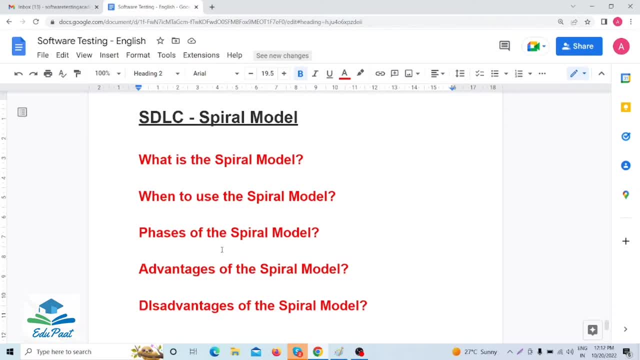 any feature of an application. that is nothing but module. okay, so when we follow the spiral model, when the modules are dependent with each other, when the modules are dependent with each other, if there is any dependence with the module, then we will follow the spiral model. right, so what is? 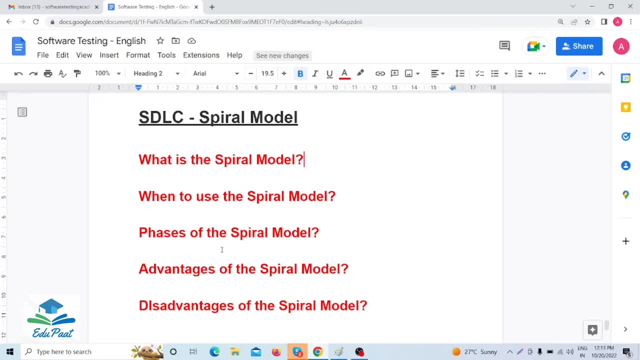 what is module? module means we can say that any features of an applications, any feature, that is nothing but a module. and what is mean by dependency? dependency means when one module is dependent with another module, that is nothing but a dependency. suppose just, for example, there is a two module, one is module a one. 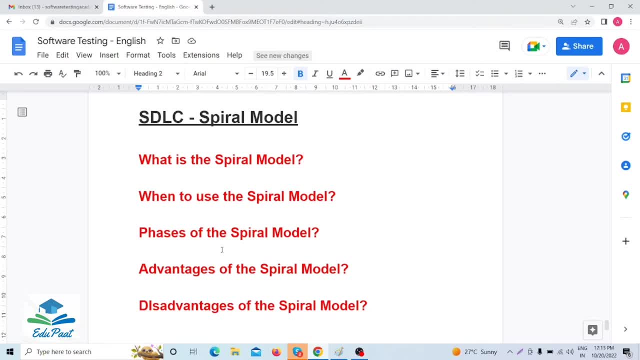 is module b, let's say module a, the name is sign, register, register page and module 2 is, let's say, login. so if anybody, if anyone is not registered, that means he cannot log in, because for the login purpose we use the registered email id and password. that means module 1 and module 2. 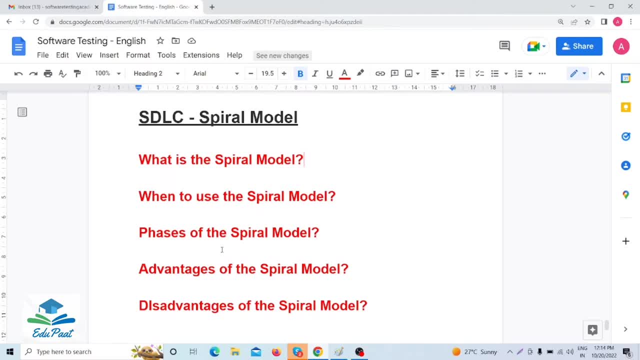 so if the Academic zeit развises using the registered, or we can say that registered page and login page, both are dependent with each other. okay, so in when we follow the spiral model, if any modules, if there is any dependency of the modules, then we follow the spiral model. now i will give you some. i will 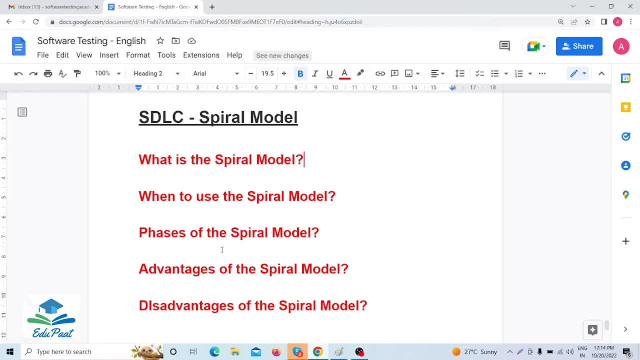 give you one example or i can tell you some phases of water model, but in a very easy way. so guys, follow my lecture one by one, so you will. you will be a good knowledge of, and meet other students. lecture one by one, so you will. you will be a good knowledge, or enum knowledge, that what is? 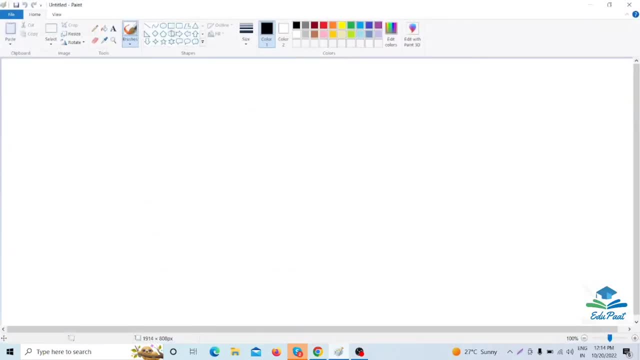 happening on the spiral model. let's say just, for example, what is the phases of spiral model? i'm telling you, suppose the diagram will be like that. so four, four divide. partitions are there, one is i'm, give, i, i'm, i'm, i'm writing the name of that phases. first phase is that this one is. 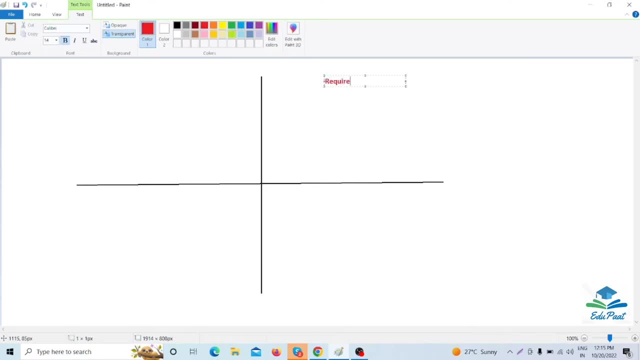 requirement, requirement collection, class and we can tell that it is study: okay, feasibility study. the first. this is the number one, phase one is requirement collection and feasibility study- okay. the second one is that design and the third one is that coding or implementation, the same as we have seen for the sdlc waterfall model. like that coding or. 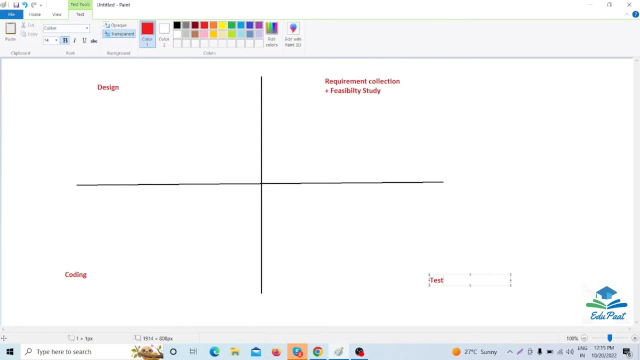 implementation and the number. last one is that testing. this is the four stage. four phases are there on the spiral model. so how spiral model work, why the num is coming to the spiral model. why the num is name is uh, uh showing uh. why why? why we call the name as a spiral? because after 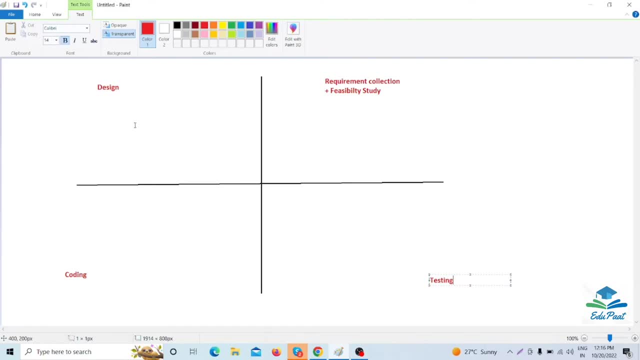 getting all the steps one by one completing, then it's look like a spy spider net. so that's why the naming thing is: looks like a pirate spiral model. okay, so yes, i'm, i'm, i'm just writing or giving some example of that. so now let's say: 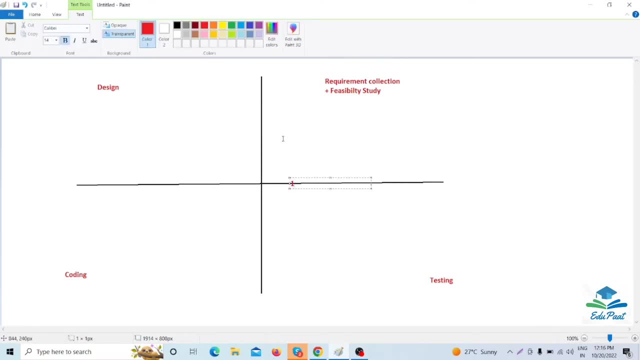 now, let's say one module has started. let's say one module has started, this is the module one. after getting the first four regs, 19 uh will will do the design, then after design, then development team will go for the coding and after coding and the coding or developing is done. 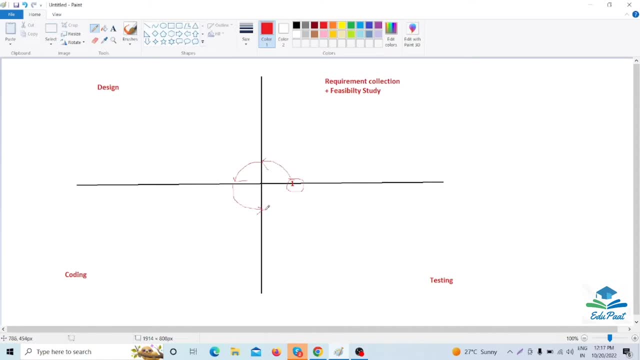 then they will assign that module. the testing team- now testing team- will check the requirement or will check the module if testing team gives the signing up or after testing the module. if that is passed, that means that software will deploy the live or we can release to that call customer or we. 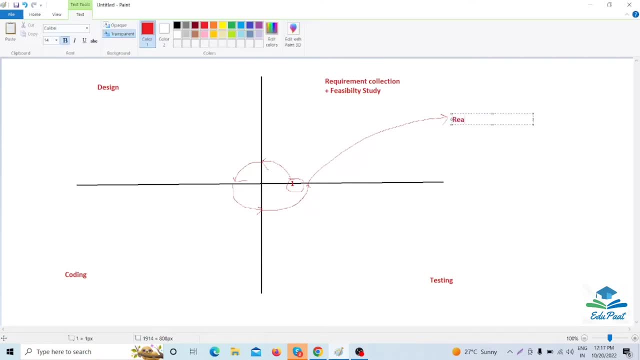 can reduce that software to the customer, let's say release the release to the customer. right, that means what is happening on that module viral model. first the module games. now after, after, the requirement collection or feasibility study will be done. when it will be done, done, then design part will be here after designing, then coding part, after coding it will be testing. 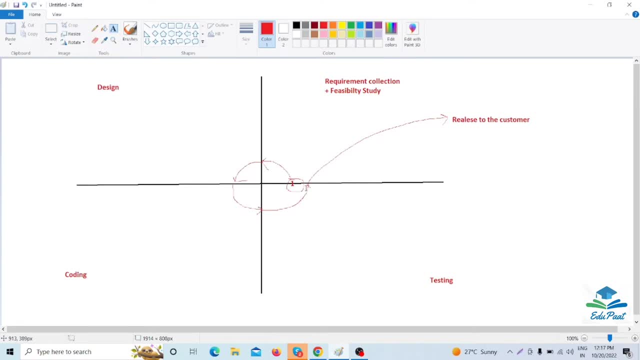 part when the testing will be complete, if there is any, if the testing will be passed, then we can release that to the customer. so that is the first module. that is the first module. so this is done. let's say this is done. now the second module coming to the picture. now the second module is: 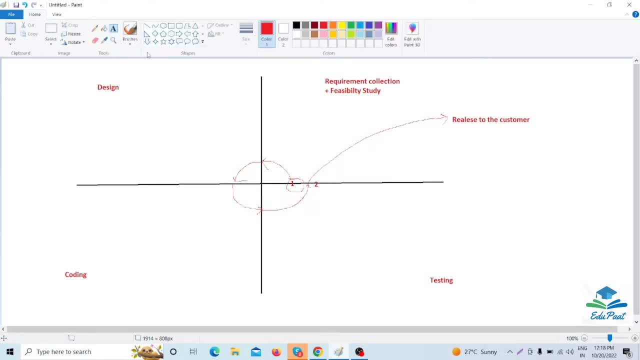 there. let's say this is the module 2. after getting the, after taking the second module, the same, the same cycle will be happening, like first requirement collection, will collection and feasibility study will be done. then, after the requirement collection and feasibility study, then designing part will be. 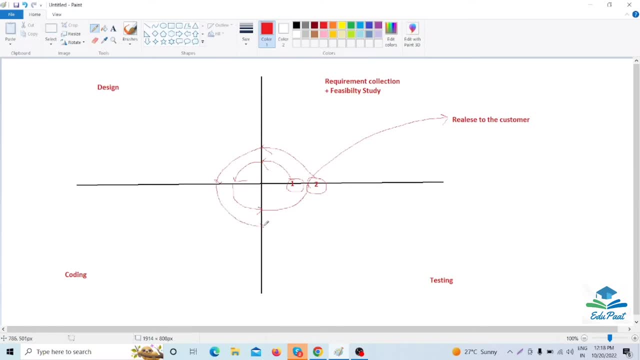 done. after designing, then coding, after coding, it will be go for the testing. if testing is passed, if the, if the software is the application is working as per the requirement, then we release to the customer. now the thing is that now here module 2 is in the picture and the previous was module 1. so what will be happening? 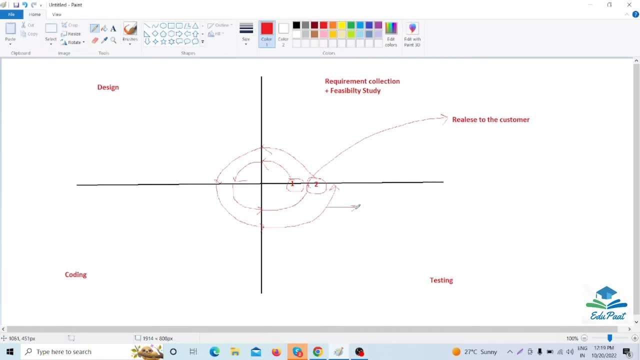 on the testing phase. what will be happening on the test? how can we test? so that is the main thing. how can we test first, first, first what? what we will do? first we have to test the module. first we have to test the module 2. okay, first we have to test the module 2, that means this module. 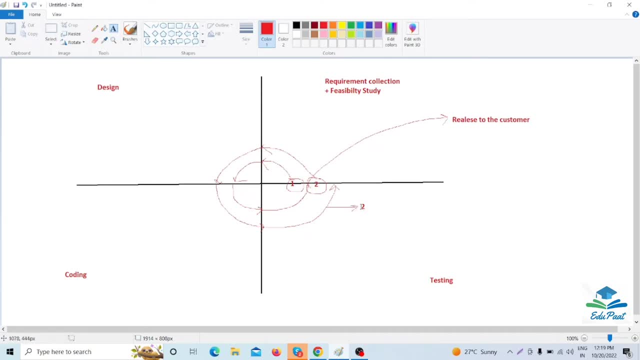 so after getting, after finishing the testing of the module 2, then we will test the integration of module 2 and module 1. that means second step will be entry integration. integration of, let's say, module 1 plus means first we have to test the module 1. that means module 2. this is the new module. first, 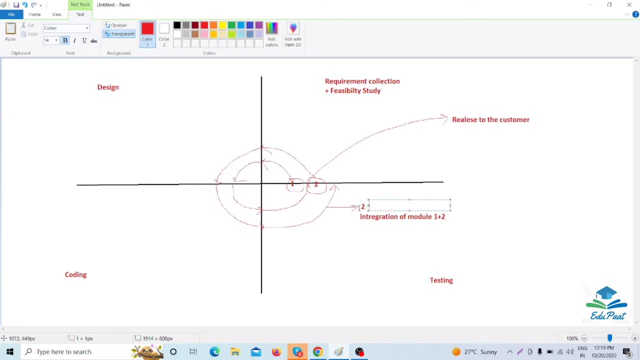 we have to. first we have to test the module 2 after completing the module 2. then we have to integrate the module 1 and module 2. that means the testing will be the integrations of module 1 plus module 2. why? why we will test module 1 plus module 2. why we will test module 1 plus module 2. 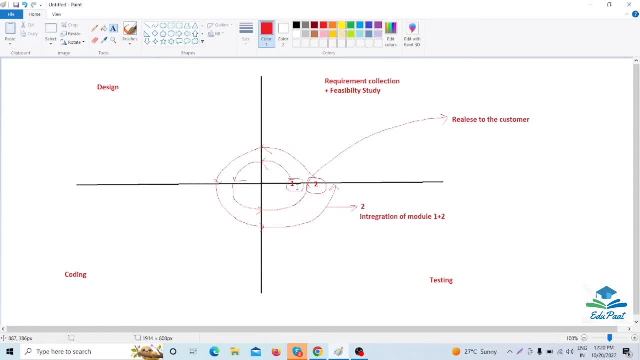 one plus module two integration. because after finishing the, after testing the module two, if the module two is perfectly fine, working perfectly fine, then obviously we have to check that after implementing the module two, is there any impact is happening on the module one or not? that purpose we have to indicate both. two means module one and module two that will be working perfectly fine, or 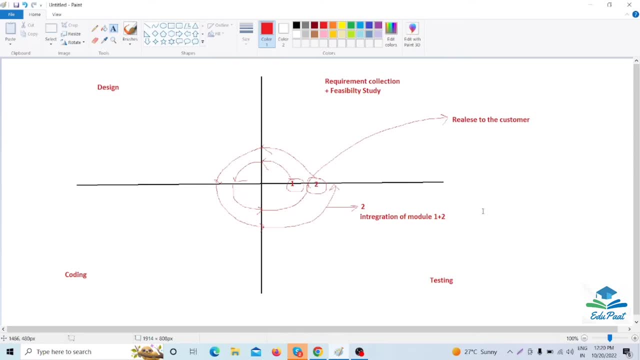 not that have we have to check. so there, module one and module two will be first, then the last, when last testing will be the, the old module. the old module means module one, the old module one. so that means for the two modules we have to test like three ways. like first we have to test the new, 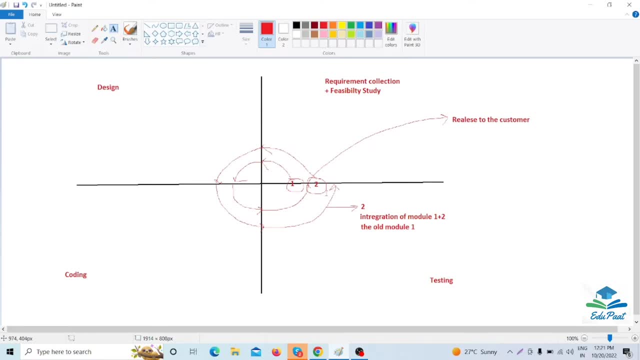 module. if the new module is working perfectly fine, then obviously we have to integrate that module one and module two means module new module and old module. and if the integrations of module one and module two is working perfectly fine, then obviously we have to test the very first module means very old module. 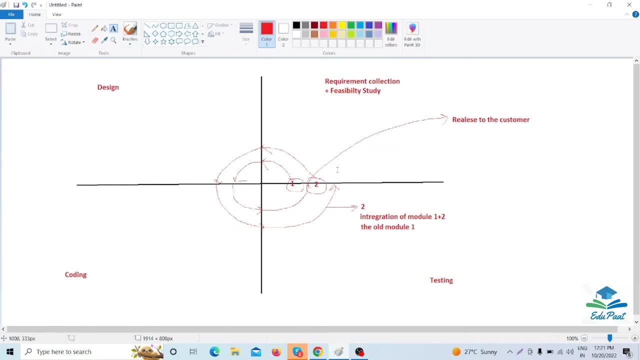 so that is the way now. if let's say, let's suppose if there is number three, number three module has coming to the picture, so the three module is coming to the picture, how it will you work? first, video common collection and feasibility study will be done. if that is working perfectly fine, in the designing the part will be: 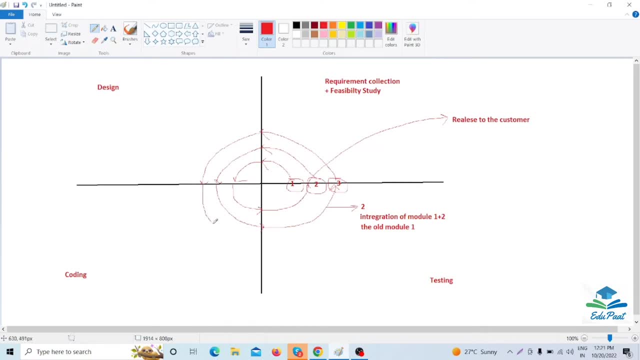 done and if the designing will be done. the designing is perfectly fine. in the coding part and after coding, what will happen? a testing part now in the tasting part for module 3, how it will be a test. there is a way first for what I have, what I have told you, that for the module to first have to test the new module like. 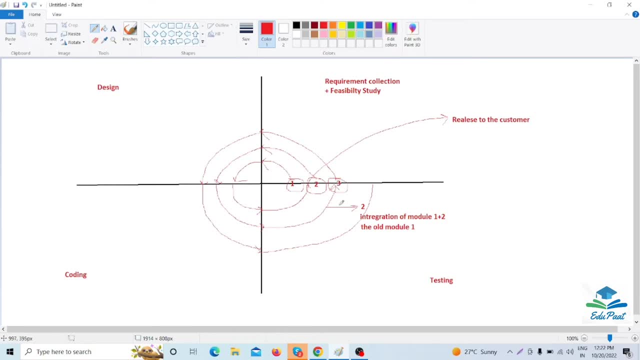 that when the new module, means the third module, is coming to the picture, then what we have to do, we have to test like that. first we have to check the module 3, very first module. what is that? 3, module 3, we have to test. if the module 3 is working perfectly fine, then what we will do, we will integrate that module 3. 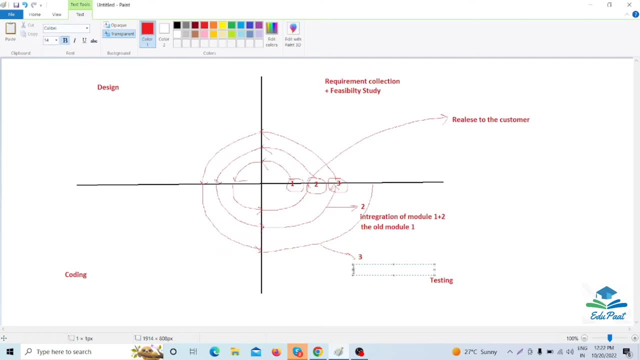 plus module 2 means first module, i mean new module, and before that i mean the last previous module. what will that then? we have to integrate the module 3 plus module 2. we have to integrate the module 3 plus module 2. so if the integrations of module 3 and module 2 is working fine, then what? 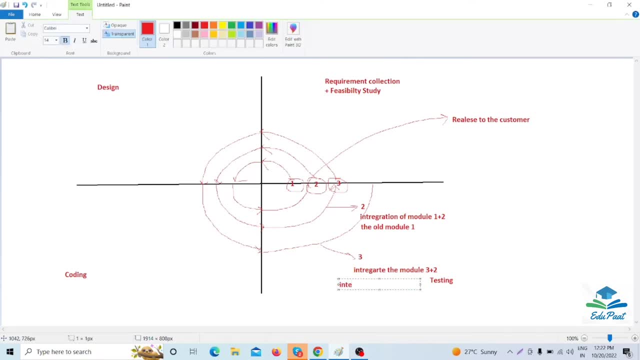 we have to do? we have to do integrate. integrate of module 3 and module 2 is working. fine, then what we have to do? we have to integrate the module 3 plus module 2 plus module 1. right, that means the new module. we have to test first if the new 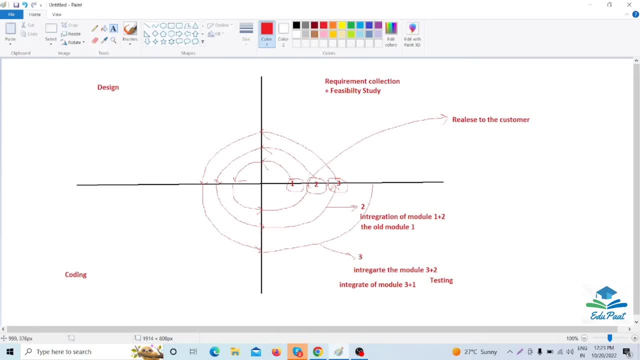 module is working perfectly fine, then module 3 plus module 2 we have to integrate and we have to test that. if the module 3 and module 2 integrations are working perfectly fine, then we have to integrate the module 3 and module 1. 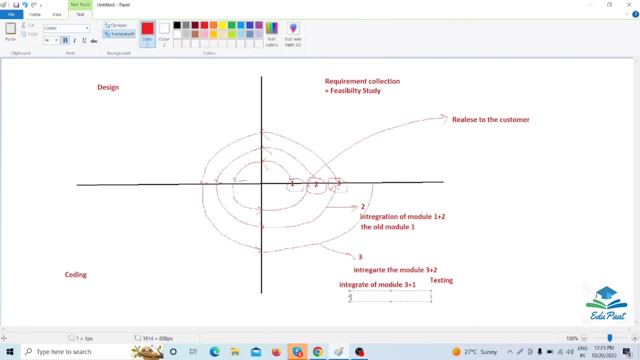 if that is working perfectly fine, then we have to test very old module, very old module which is nothing but module 1. we have to test the module 1, right? so, like that, we have to test very old module. we have to test module 1, obviously, as the module 1 is there. so we have to. 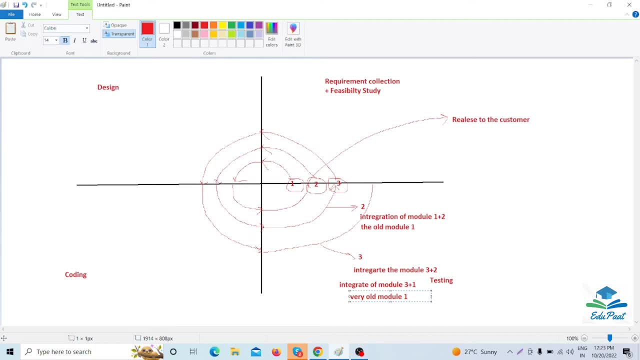 test the integrations of very old module which is nothing but module 1 plus module 2. that means, for the third module we have to. how will? how we will test. first we have to test the new module, then we have to integrate the module 3 plus module 2, then again we have to integrate the module 3. 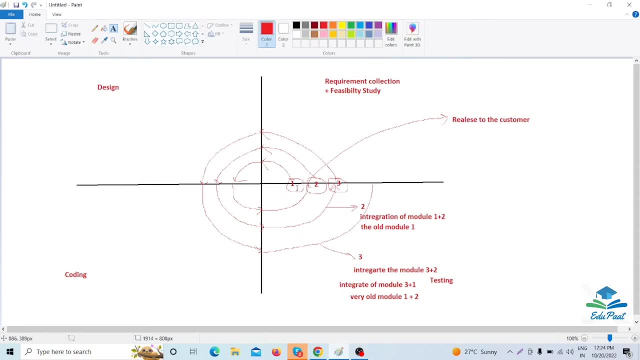 plus module 1 and that, and if that is working perfectly fine, then we have to test the very old module, which is nothing but module 1 plus module 2 integration that we have to test. so like that it will be work if the all our module is working perfectly fine. 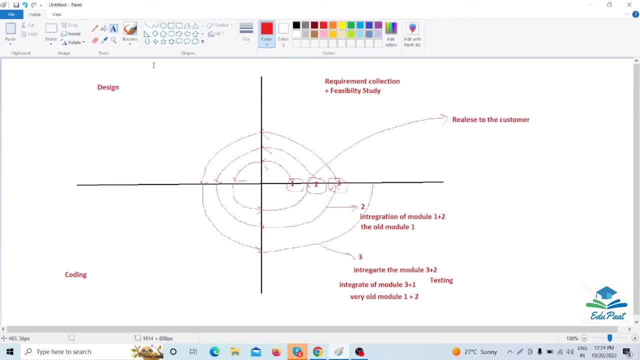 then we have to release that module, then we have to release the module to the customer right. same for the module 4, same for the module 5 if there is nth number of module are there. so the process will be the same. so now, i already told you that. why the name is spiral model? i told you. 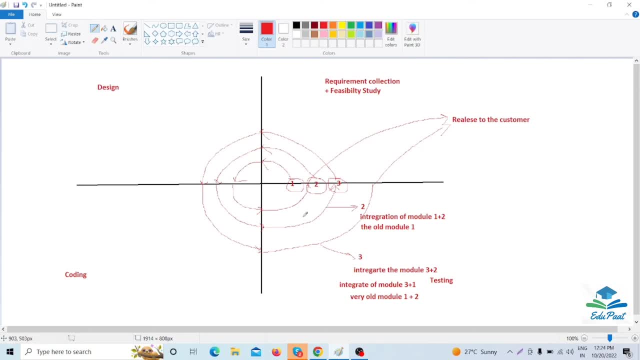 that it's look like a spiral net, spider net. so you can see that it's look like a spider net. so that's why the naming is that spiral model. so now we can say the spiral model, also called as a iterative and incremental model, we can say that spiral model is named as a iterative. 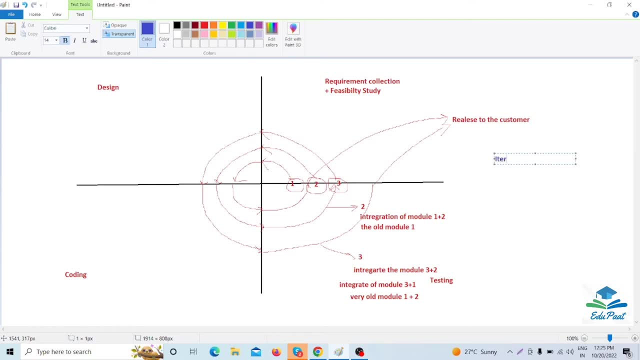 iterative model. we can say the iterative model and we can say that in, in, in, in, in, in. incremental model, incremental model. so why the spiral model is called as a iterative and incremental model? because why the name is as a iterative model? because we perform the same process in each cycle. 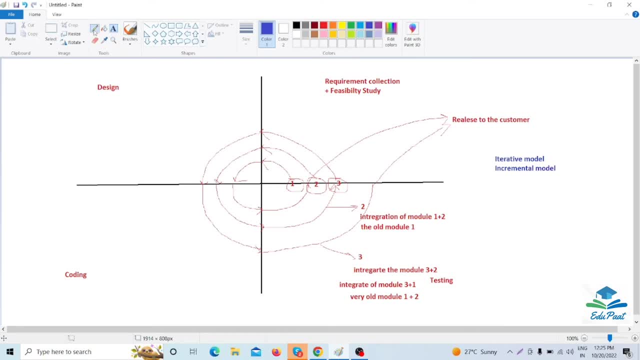 we perform the same mode, same process, in each cycle. we can say like that: perform fats, the fences, in each cycle, in each cycle. be performed the same process in each cycle. that is why the scaling is the iterative model, so as we can see that we are from the same process in each. 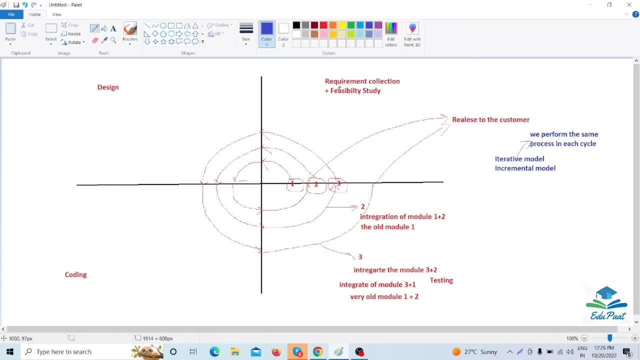 cycle so up. so the first Sunshine collection plus feasibility study to the testing part. so that is one cycle. so that this is one cycle. this is the one cycle. right then? this is for the module 2. this is the one cycle and module 3: this is the. 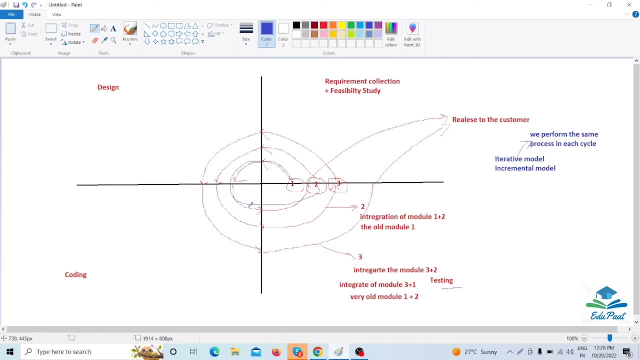 one cycle. so why the name is why? why we can say spiral model as the iterative model, because we perform the same process in each cycle. so that's why the name is the name is iterative model and why we can say it the incremental model, because modules are keeps on increasing. we can see that. 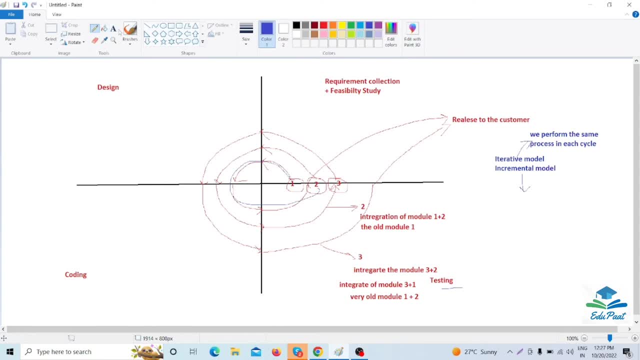 modules are keep on increasing, so modules are. modules are upon increasing. modules are keep on increasing now, so we can test up to nth number of module. there is no limitations of module. as for the client's requirement, if the client has the n, number of module is there, so we have to test one module to. 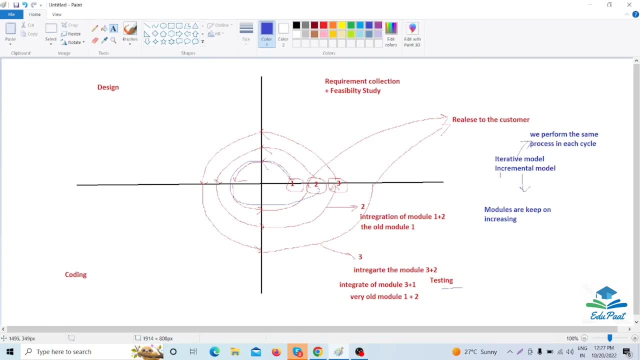 nth number of modules. so that's why why the name is the incremental model, because modules are keep on increasing. so that's why it's the naming is the incremental model. we can say that we can. spiral model is also called as a iterative models and incremental model. now you guys have a clear. 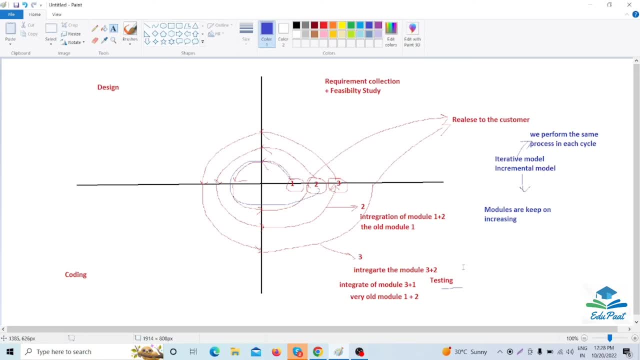 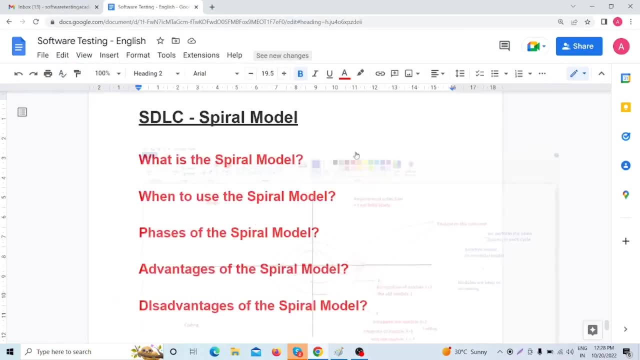 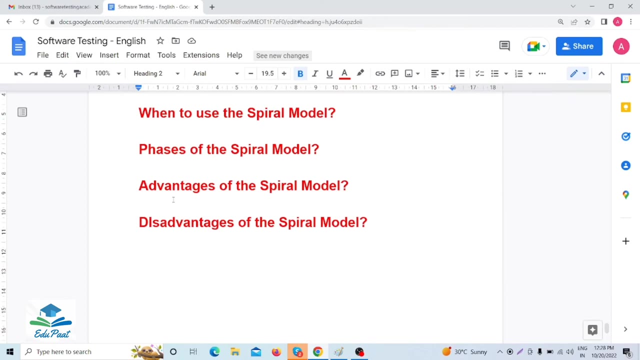 idea, clear picture that what is happening on the spiral model and why the naming, why the name comes to the picture as a spiral model. okay, now i will give you some advantages of spiral model. what is the advantages of spiral model? so here i mean in the spiral models, requirement changes are allowed. 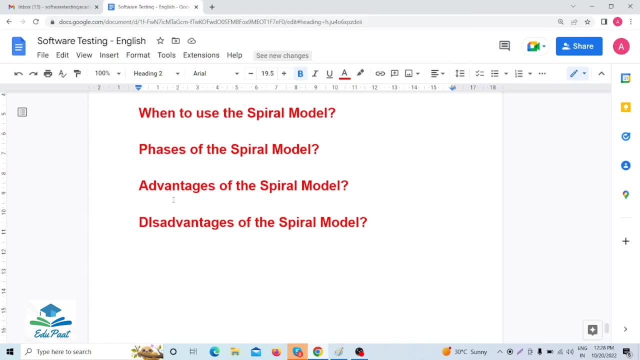 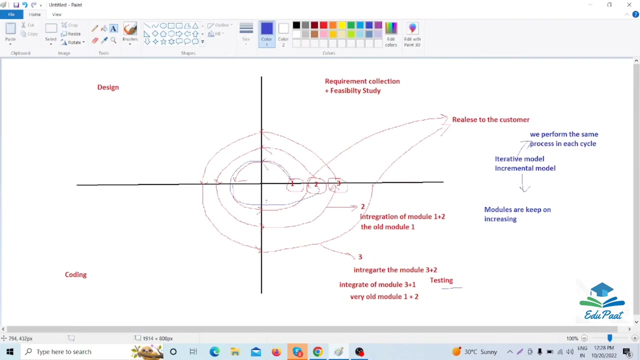 after every cycle, requirement changes are allowed. i can write this thing: requirement changes are allowed are allowed after every cycle. now, requirement changes are allowed after every cycle means means: so that is one cycle. so what will be happening on the waterfall model? if we change the model, we change the phases, then we cannot revert back. 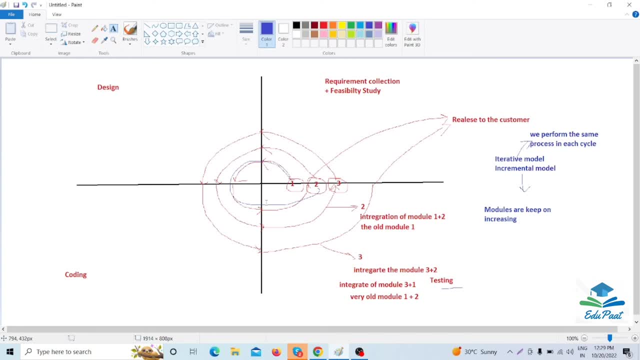 so there is no changes of requirement done. all the things will be done on the only maintenance part. that means after deployment, in the maintenance phase we can change that. but in the requirement in the spiral model after every cycle we can change the requirement. that means requirement changes is allowed after every cycle. so that is the most most important advantage of the spiral. 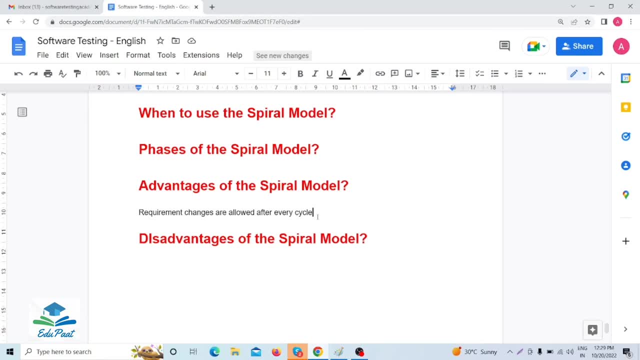 model requirement. changes are allowed after every cycle. and the second advantage: suppose we are working in a module or we have worked in a module. let's say that is completed, we have worked in a module and that is completed, then we have released that module or we have released the software to. 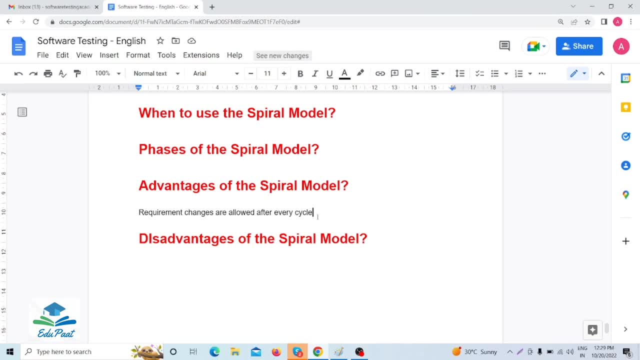 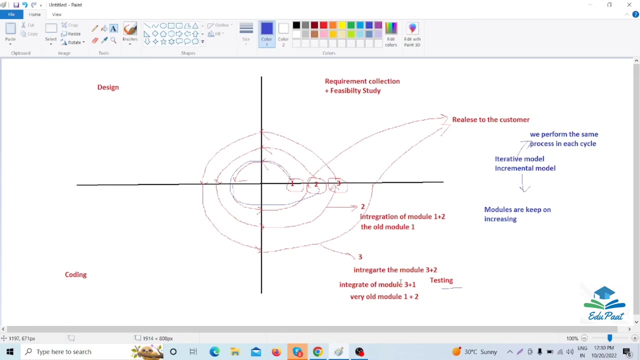 the customer. that means we can say, after one module complete, then we can take the second module. so what will be happening in that? so that is module one: requirement collection and feasibility study is done, designing part is done, coding part is done, testing part is done. after completing all the phase, if all, 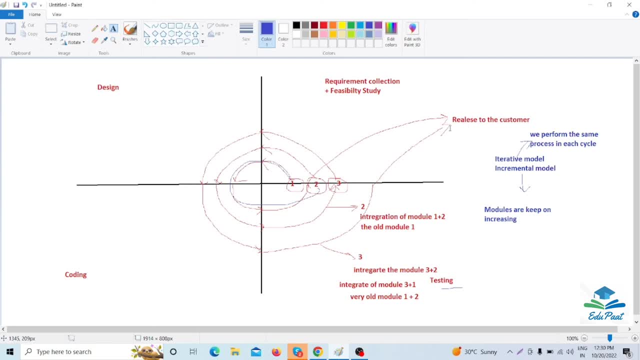 are working perfectly fine, then we release to the customer, then we release to the customer and after release to the customer then we take the second module. that means after one module completion then we can take the second module. so that is the most, also one of the advantage of the. 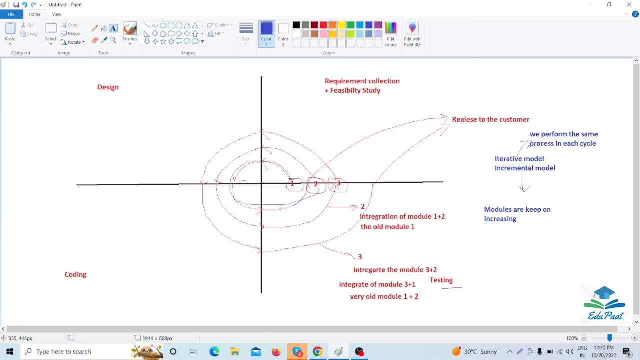 spiral model. so after completing one module, then we can take the second module for the new implementation. so this process is nothing but called nothing but called a control model. so after completing one module, then we are taking taking the second module. so that's why we can say that is the control model. 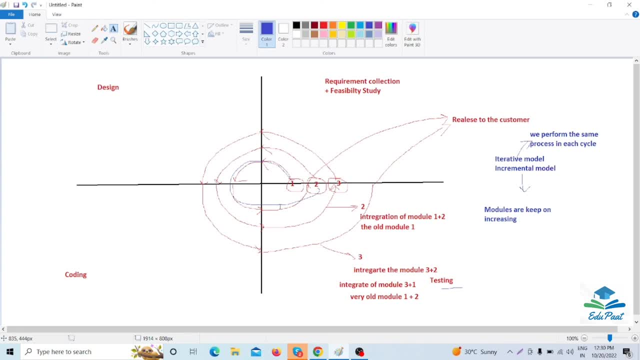 also okay. so these are the advantage of the spiral model. so what is the first advantage here? requirement changes are allowed after every cycle- and the second second advantage is that suppose we are in where we have worked on a module and that is completed and we release that module to.